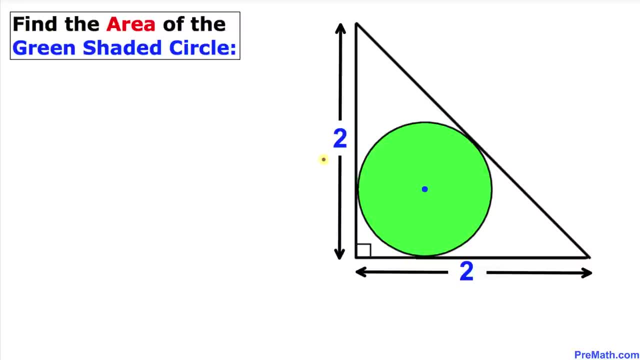 Welcome to pre-math. In this video tutorial, we have got this right angle isosceles triangle and in this triangle we have got this circle that is inscribed in it and, moreover, the side lengths of this triangle are two units each, and now we are going to find the area of this green. 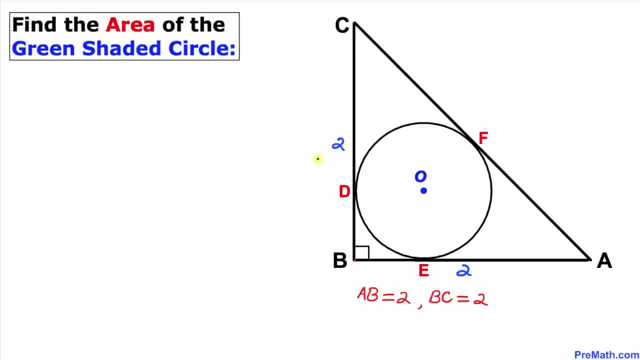 shaded circle. So let's go ahead and get started with the solution, and here's the very first step. Let's focus on this triangle ABC, and over here in this triangle, we know that this side AB is two units and this side BC is two units as well, and since this is a right triangle, therefore we 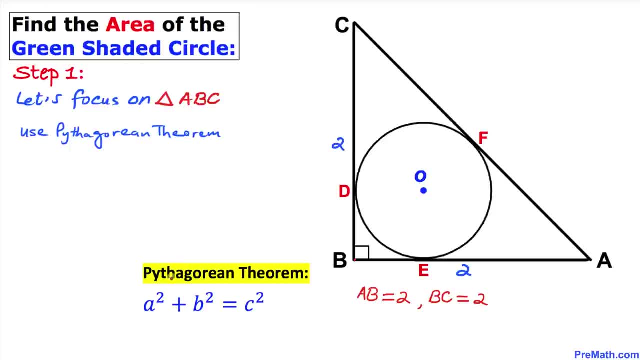 are going to use the Pythagorean theorem. and here's the Pythagorean theorem: A square plus B square equal to C square. In our case, the longest leg is AC. I'm going to call this side C. This horizontal side of this triangle, I'm going to call A, and this vertical side, I'm going to call: 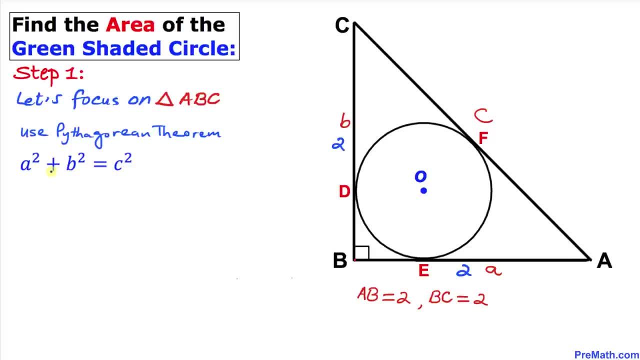 B. and here's our Pythagorean formula. Let's go ahead and fill in the blanks: A, in our case, is two, so that's going to become two square plus B, in our case, is two again, so that's going to become two. Two square- equal to C square, So two square is four plus four equal to C square, So C square is: 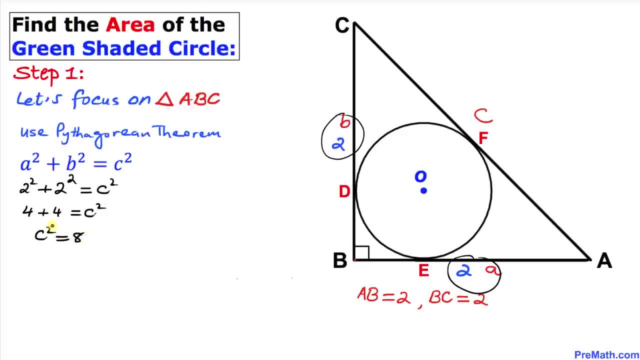 going to give us eight. Let's take the square root on both sides to undo this square. So C is going to be simply square root of eight. and now you can see this square root of eight. I have just copied it down and I just simplified it. and the reduced and the 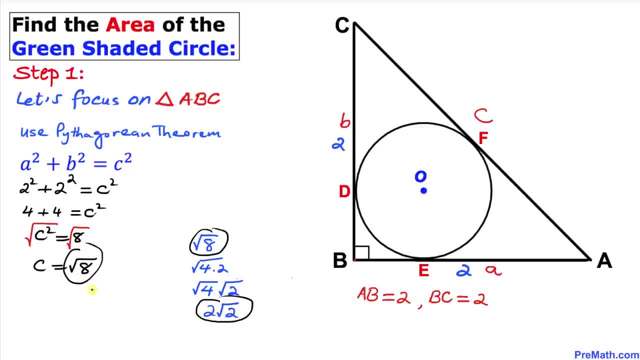 simplified form is going to be a two times square root of two. So I can write this: C equal to two times square root of two, and we can see that this side C is same as this distance, AC. so I can write this one as AC equal to two times square root of two. and here's our next step. 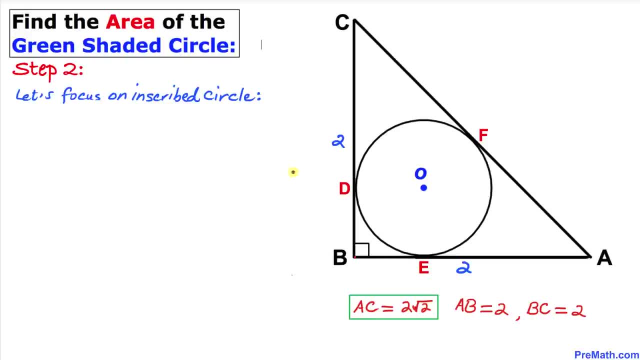 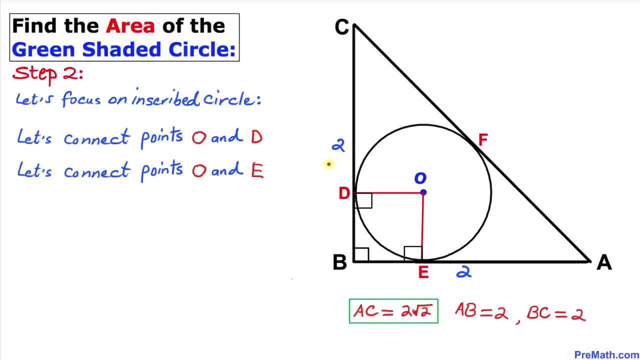 let's focus on this inscribed circle. let's go ahead and connect points o and d. so let me go ahead and connect that one, o and d, and likewise we are going to connect point o and e, and here's our much nicer looking diagram. let me call this radius as lowercase r. therefore od equals to r. 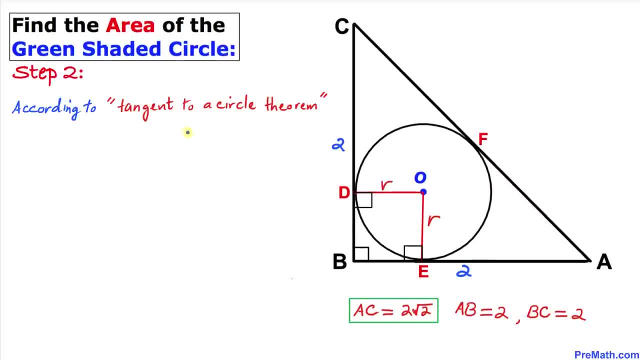 and o e equals to r as well. now let's recall tangent to a circle theorem. and here's a tangent to a circle theorem. the angle between a tangent and a radius is always 90 degrees. that means they are perpendicular. in our case, this radius and this tangent line, they have a 90 degree angle. 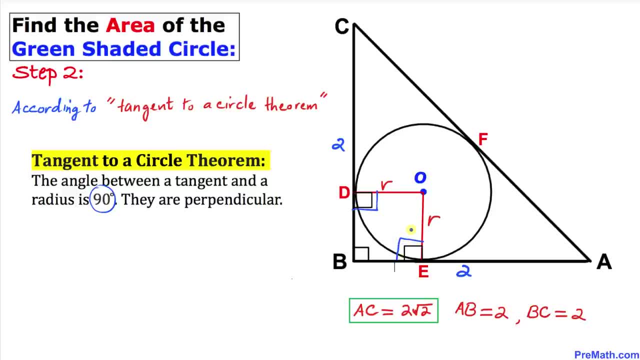 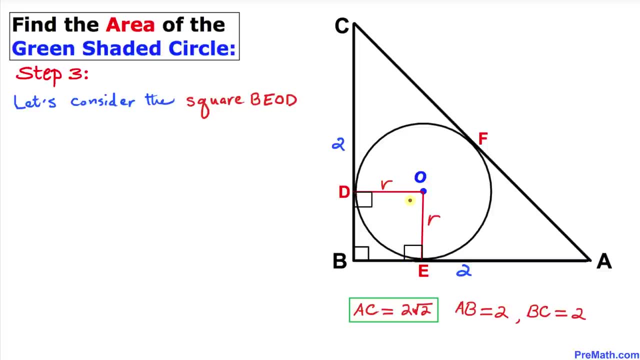 and likewise. this one is 90 degree again. and here's our next step. let's consider this square: b? e, o, d. here's the definition of a square. all side have equal lengths and every interior angle is a right angle. that means 90 degrees. therefore, this b? e equals to r, and likewise. 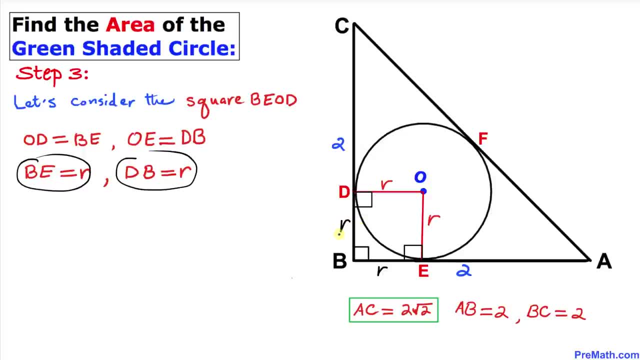 d b equals to r as well. let's look at this. a b distance is 2, isn't it? and this b e is r, so therefore, this distance e a is going to be 2 minus r. thus our e a distance is 2 minus r. now let's look at the. 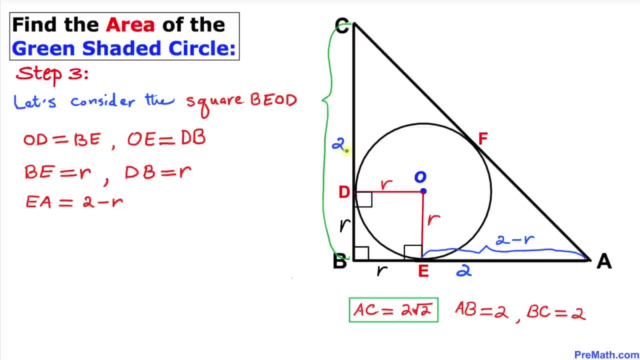 other side, this b c. we know that this total distance is 2. we know this b d is r, then this distance c d is going to be 2 minus r. so the c d distance turns out to be a 2 minus r as well. and now, in this next step, let's recall this two. 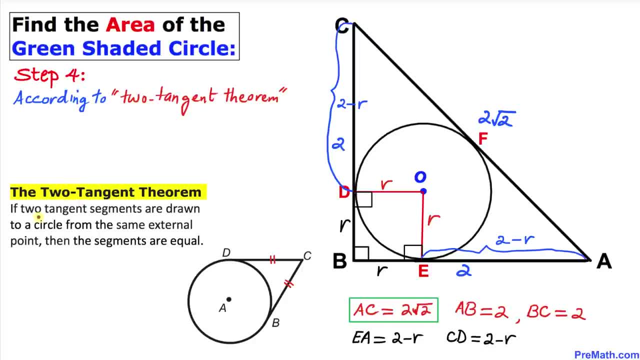 tangent theorem. and here's a two tangent theorem. if two tangent segments are drawn to a circle from the same external point, then segments are equal in length, as you can see in this figure. so therefore, according to this theorem, this tangent line is going to be equal to this one. 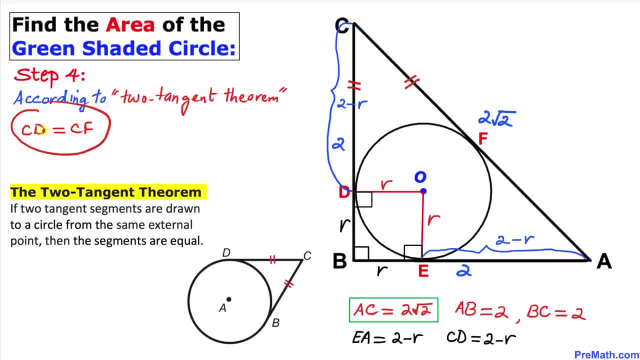 no wonder i put down cd equal to cf, and since cd is 2 minus r. so therefore this cf is going to be a 2 minus r as well. and likewise, on this side, this tangent e a is going to be equal to af. and since e a is 2 minus r, then 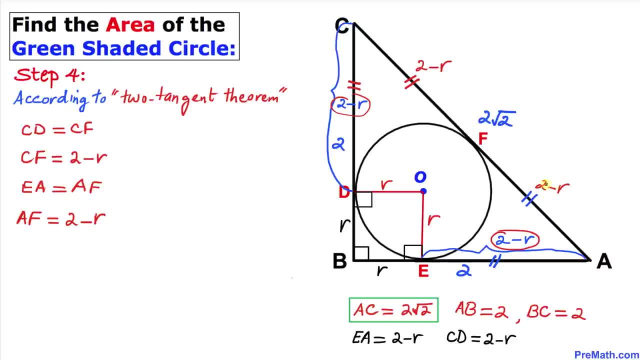 is going to be 2 minus R as well. now let's focus on this line, segment AC, which we can see equal to this CF and then plus AF, isn't it? so in our case, CF is 2 minus R and AF is 2 minus R as well. so let's go ahead and simplify in our 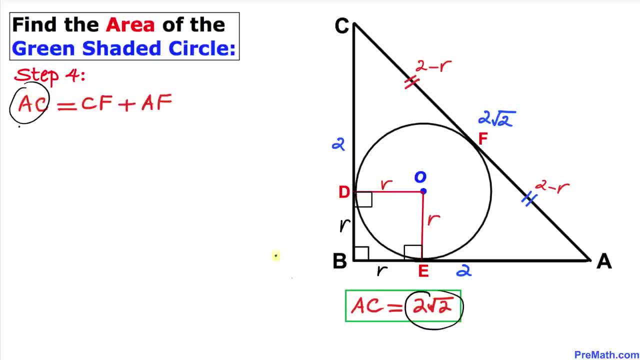 case, AC is 2 times square root of 2. let's write down: 2 times square root of 2, equal to CF, in our case is 2 minus R, plus again AF is 2 minus R again. let's simplify: that's going to give us 2 times square root of 2 and here 4 minus 2. 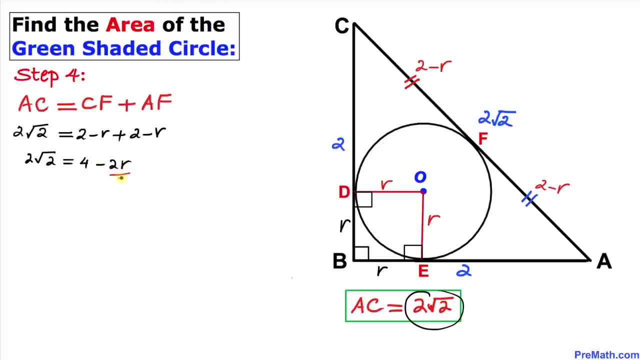 R. let's divide across the board by 2 to make things simple. so that is going to give us: square root of 2 equals to 2 minus R. that means R value is going to be simply 2 minus square root of 2. and here's our final step. let's recall the area of a circle formula and here's a. 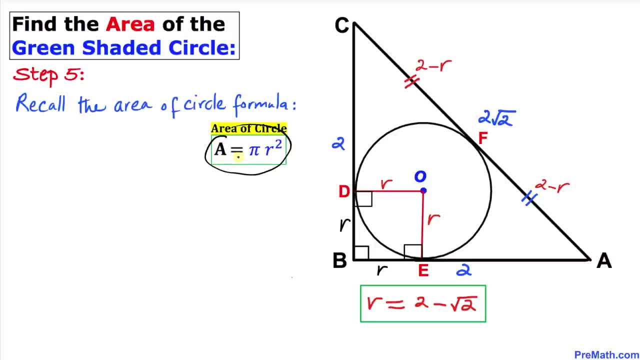 circle formula: a equal to PI R square where R is 2 minus square root of 2. let's go ahead and fill in the blanks, so area equal to PI times 2 minus square root of 2 and then square. now let's focus on this.